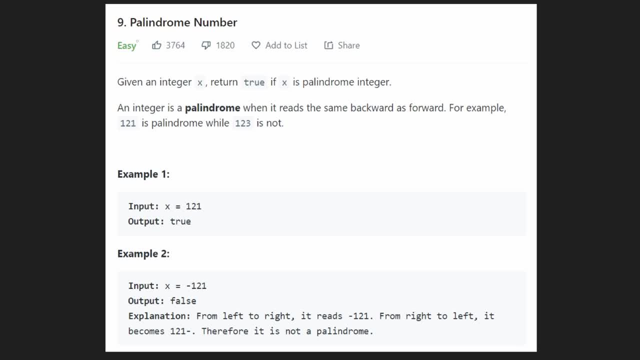 Hey everyone, welcome back and let's write some more neat code today. So today let's solve the problem: palindrome number. In this problem, we're given an integer x and we want to return true, if, and only if, this integer x is a palindrome number. And what exactly is a palindrome? Well, 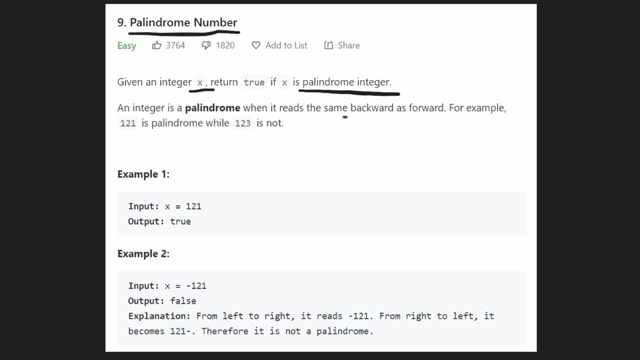 basically a number that reads the same way as it does backward as it does forward. Basically, you reverse it and it's the exact same, And you probably know. if you're familiar with palindromes, you probably know how to detect palindromes when it comes to strings. So you might think, okay, we 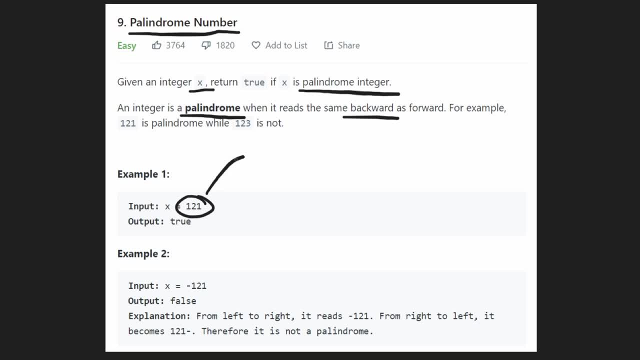 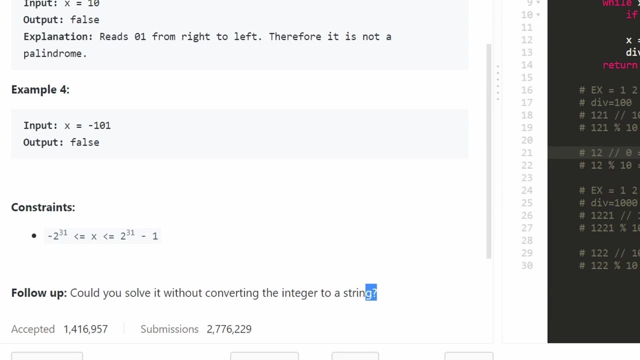 can just take this entire number right: one two one, convert it into a string like one two one, and then it'll be easy to determine if it's a palindrome. That's a good idea. but if you read down below, the follow-up question they have for us is: can we do it without converting the integer? 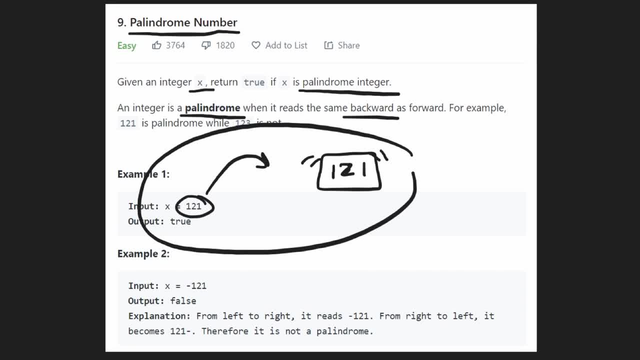 to a string. So that's going to make this problem a little bit more tricky for us, but I'm still going to show you how to do it. So with a string it would be easy, because we could have two pointers right: a pointer at the beginning and a pointer at the. 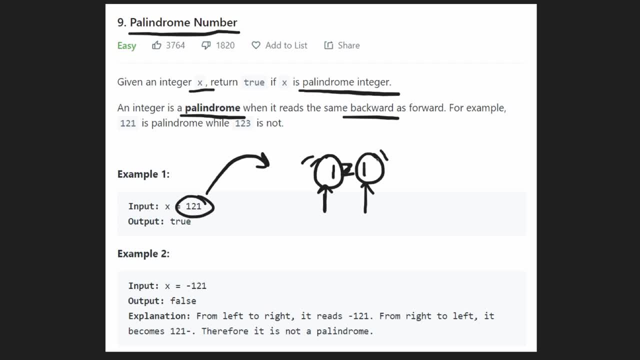 end, and then we could just compare each character or each digit, and if they're equal we continue, if they're unequal, then we return false, because then we know it's not a palindrome. Basically, I'm going to use that same idea, but I'm going to use it without creating a string. I'm going to use it. 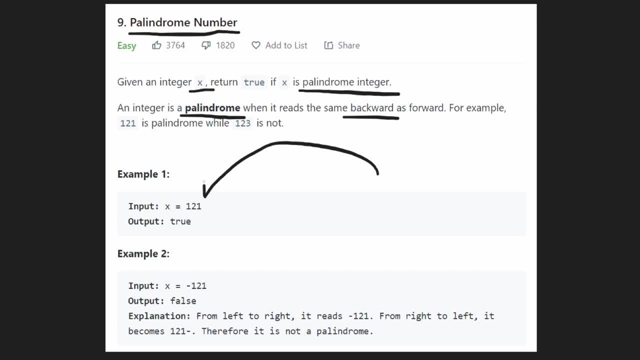 just by doing the math operations on this input integer. So suppose we have a value, one, two, one we want to know if it's a palindrome, So one. what we want to do is we want to get the ones place and get the left value right, the left value and the right value. How do we get the right? 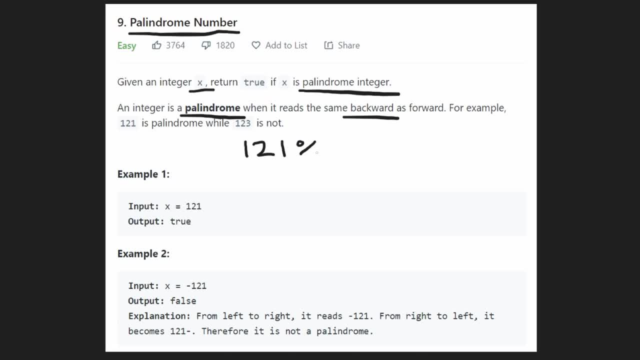 value. That's the easy part. right in math you might know from some programming problems you've done: if you mod something by 10, we get the ones place right. if you take 121, mod it by 10, we get the value 1 right, which is what we wanted to get. we wanted to get this right value. Next, what we 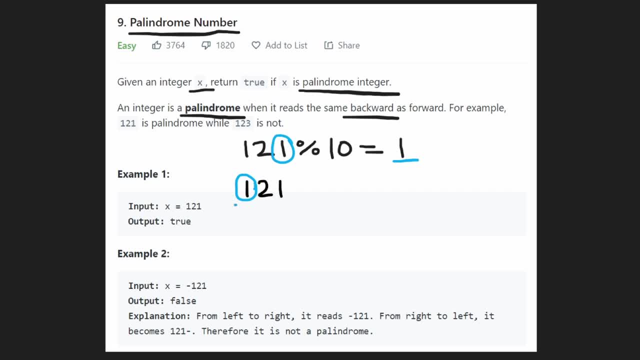 want to do is we want to get the left value. so how are we going to get this left value? because once we get the left value, then we can compare it with the right value and then we can check if it's a palindrome or not, right. Well, what math operation could we do on this to get this value? We are 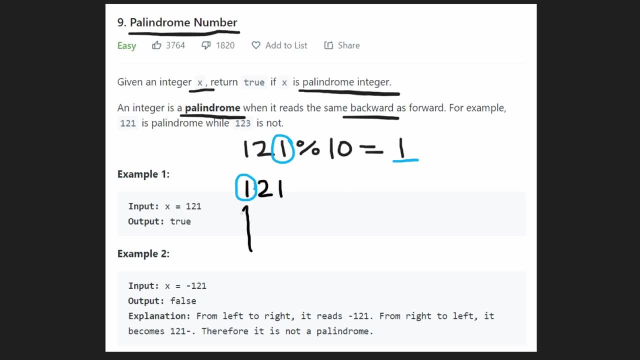 asking ourselves: this is 121. we want to know what value goes here. in other words, we want to know what digit is in the hundreds place. How can you do that in math? Well, if we divide the value by this by, by 10, not by 10, but if we divide it by a hundred, then that will tell us how many a hundred. 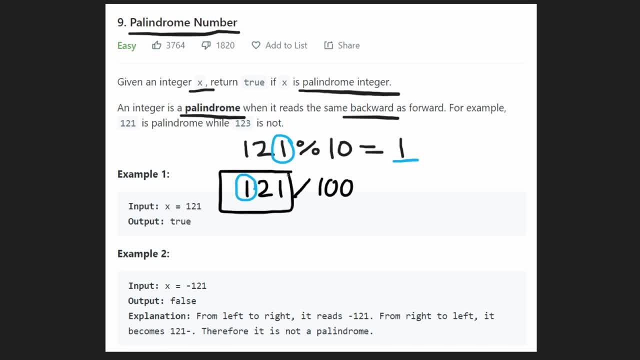 how many hundreds go in this value and it'll always round down towards zero. so in this case, 121 divided by 100 is going to evaluate to 1 because we're rounding down, right? if instead we were doing 220 divided by 100, then we would get 2 because we have two hundreds in this value, right? 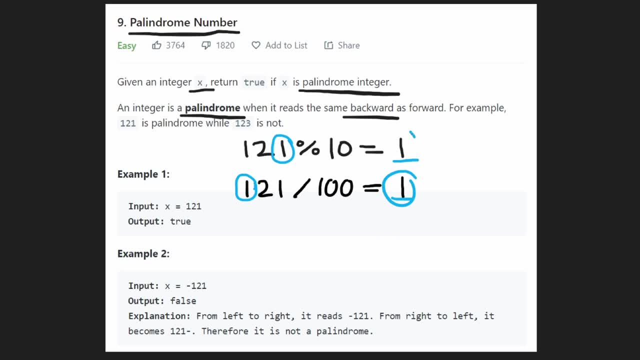 so that's kind of the idea. okay, so now we have the left value and the right value. we compare these two together. they are equal to each other. right, so then we can continue. right, but now we we compared these values, so we want to chop them off. how can I get rid of the left and right values? so if I have 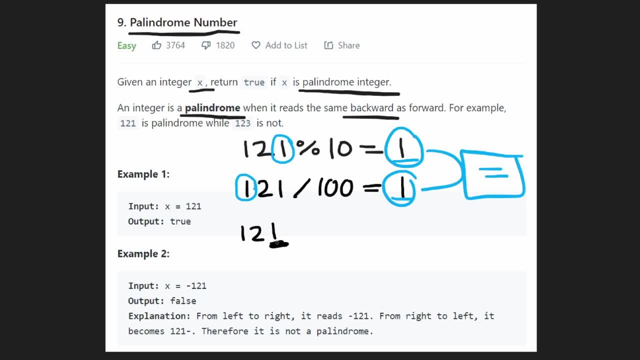 121. I want to get rid of the right value because we already compared it right. how can I do that? well, I can take this, divide it by 10. that will chop off the ones place. so if I divide it by 10, it'll round down and then we'll get the right value and then we can continue right, so now we're. 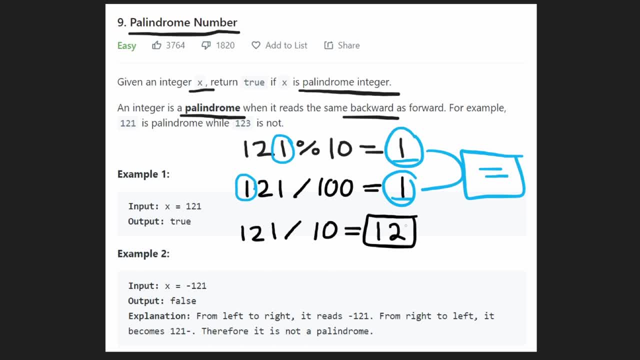 done, we'll get the value 12.. that's awesome, because that's what we wanted to do. so if we have 121 and now we want to get rid of the left digit because we already used it, how do we get rid of this left digit? well, we had a hundred up above right. we were taking this and dividing it. 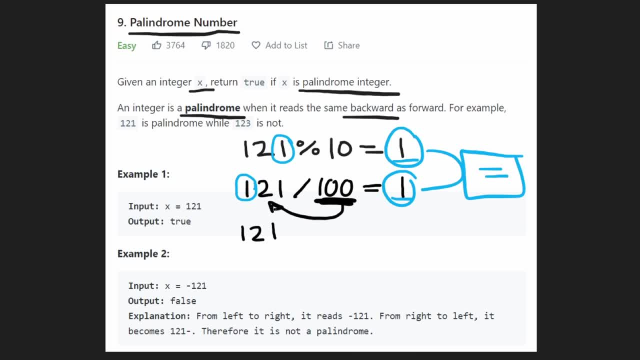 by a hundred, because we know that a hundred is the most significant digit for this right. we couldn't do a thousand because a thousand would be too big right. so if we take a hundred and actually take 121 and mod it by a hundred- and this is the kind of the tricky part that that makes this problem. 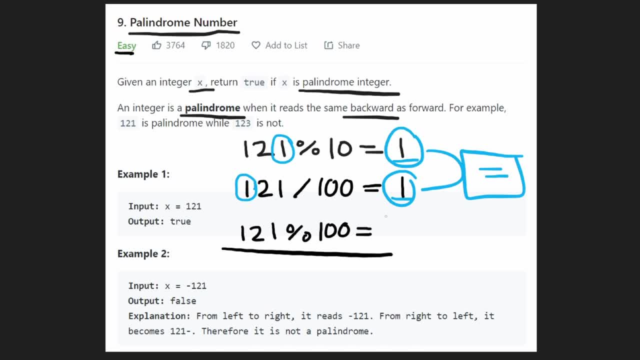 difficult, right? that's why this is a follow-up, because you probably wouldn't guess to do something like this. at least it would take some thought to figure it out, right? so if we take a hundred, it take 121. mod this by a hundred, that'll get rid of this first digit for us, because it'll 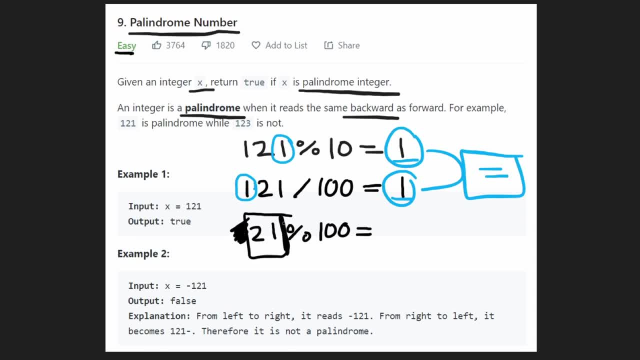 give us all the remaining stuff in this portion, right. so when we, when we do this operation, we're left with with 21, right? our goal was get rid of this one's place, this one digit, and we did that. our next goal is to get rid of this. 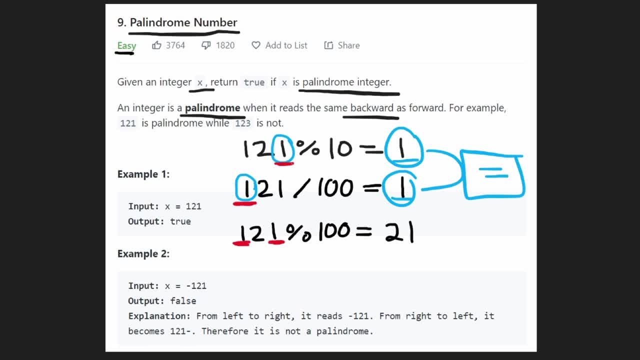 digit right, because we used this digit and we used this digit. we want to get rid of them. how do we get rid of this one over here? let me show you how. so this is the easy part. right, we have 21. if we divide 21 by 10, that's how we can get rid of the one's place right, and it'll always round down. 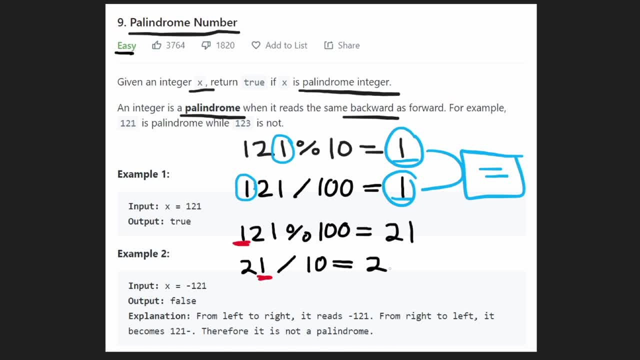 right. so 21 divided by 10 is going to be 2, because it's rounding down. so we successfully did what we wanted to do: we chopped off the left and right digits, right. so now we're left with 2, and then, now that we have our new digit or the new value, we're basically going to repeat what we just did. 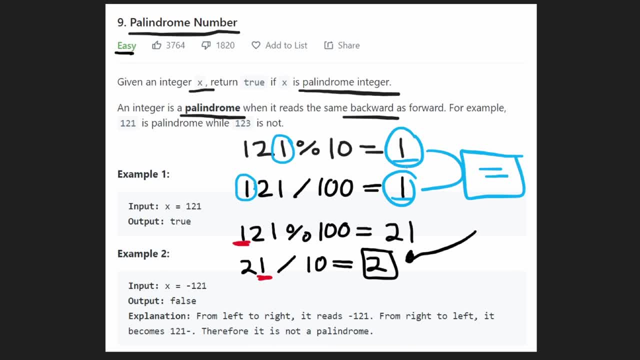 up above. except the only difference is going to be up here to get the, to get the- obviously the left and right digit. since this is just one value, the left and right digit are going to be the exact same right. so, up above, to get the left digit, what we did was we divided it by a hundred, first right. 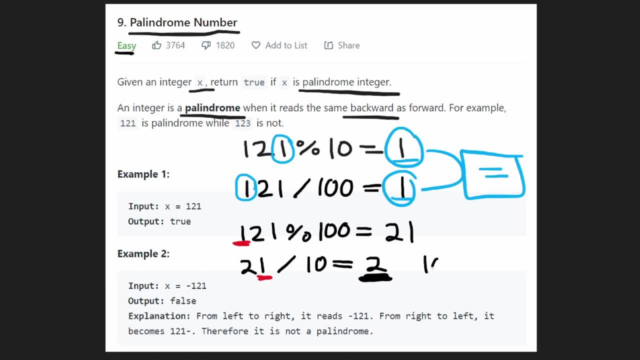 now, instead of dividing this by a hundred, we're actually going to be dividing this by one, because we chopped off two digits, remember? so before we had a value that was at least greater than a hundred. now we chopped off two digits, so now we're going to have a value that's at least greater than. 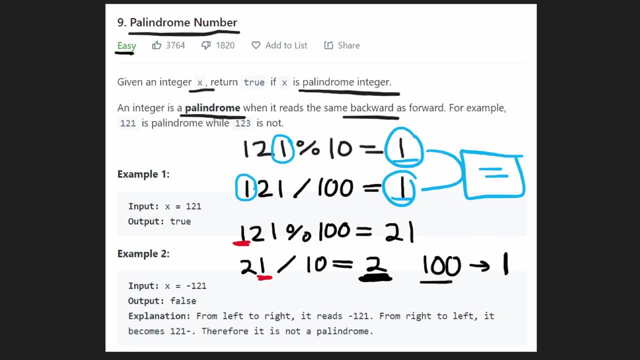 one. that's why we're, when we get the left digit, every time we're going to be taking this value and divide and basically removing two digits from it. so i hope that this makes sense so far, and let me just repeat this on a different example to give you a slightly more clear explanation, and 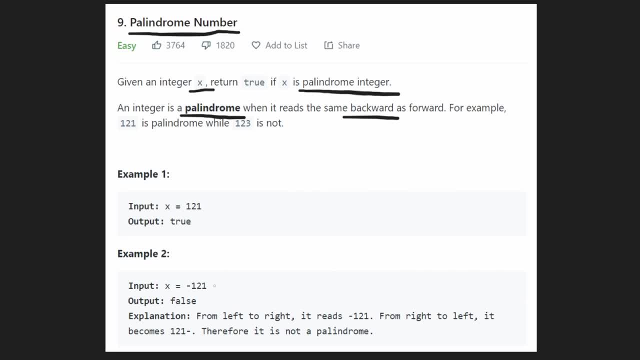 one other thing i want to mention is down below, in the second example, you can see that we have 121, except it's negative. right, so it is a palindrome, but it is negative. so negative numbers in this case are always going to be false, because you can see, once we reverse it, we have that. 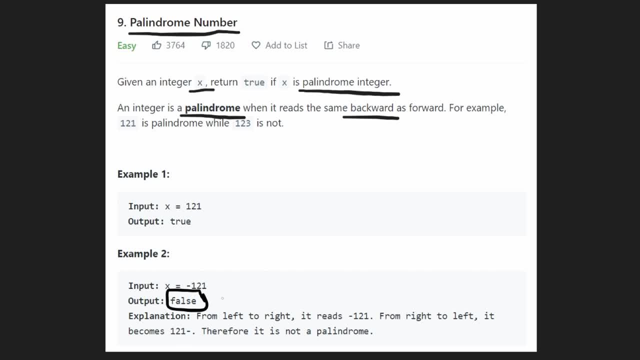 negative sign on the right side, right. so we don't want that. negative numbers are always going to be, so any negative numbers are always going to be false. now let's take a look quickly at a different example, slightly different: one, two, two, one. so this is just one extra digit. so if in this case, we want 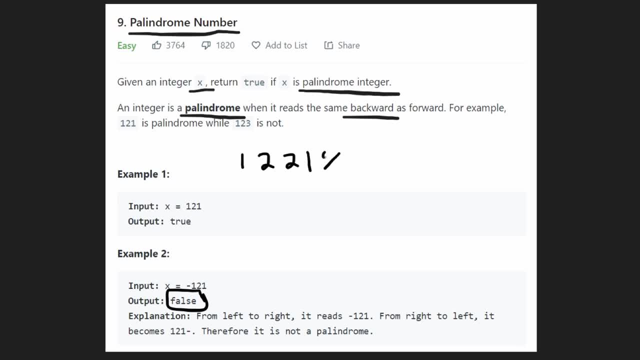 to get the right digit, which is one, once again, we're going to take this, mod it by 10. we get the one value on the right. if we want to get the one, the value on the left, we're going to take one, two, two, one and divide it by a thousand, right, a thousand, because this value is in the thousands. 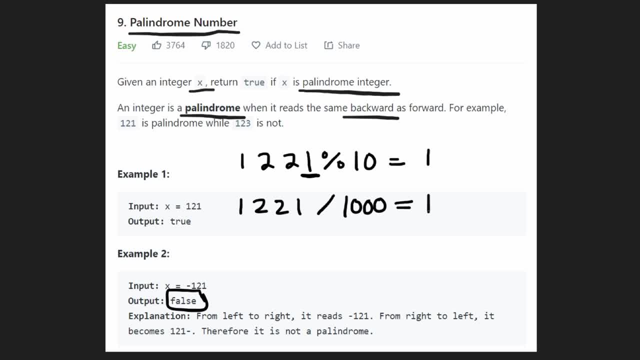 right. so we divide that and once we've done that, we'll get a one, which is the one from the left side, right. so now we compared it right. we did what we wanted to do. now what we're going to do is chop off the left digit and the right digit. so once we do that, we're going to be left with 22 right. 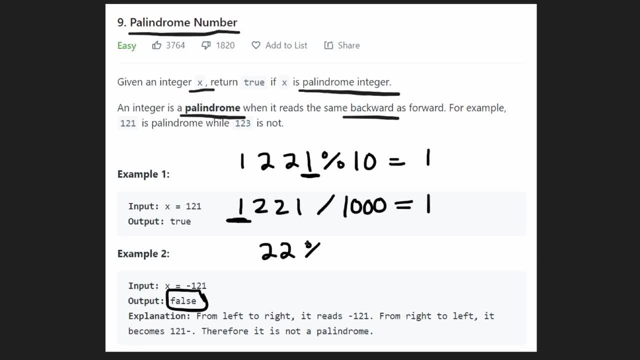 now we want to get the right digit. how do we do that? once again, just mod it by 10, right, that's what we did up above. it works this time as well. mod it by 10, we get the right two. how do we get the left two right? this case 22.. 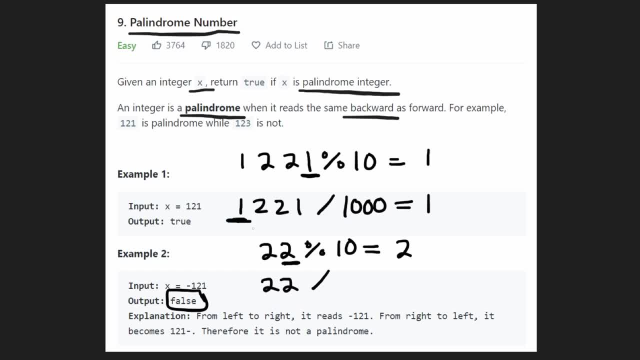 two. previously we divided this by a thousand, right. that's how we got the left digit from over here. right now we want to get the left digit again, instead of dividing by a thousand. now i'm going to divide by 10, right, instead of a thousand, because we got rid of two digits, right? so we 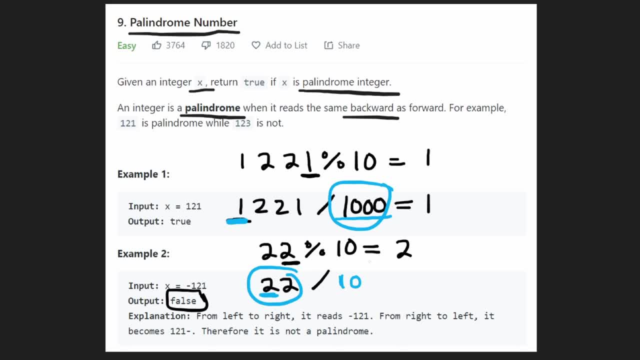 have to get rid of two digits from here. so when we take this from a thousand now, it becomes 10, and then we get that same left digit, two right. so what i'm saying is this value that we have here. it's going to go from a thousand to being 10. right before, what we had was a hundred and that. 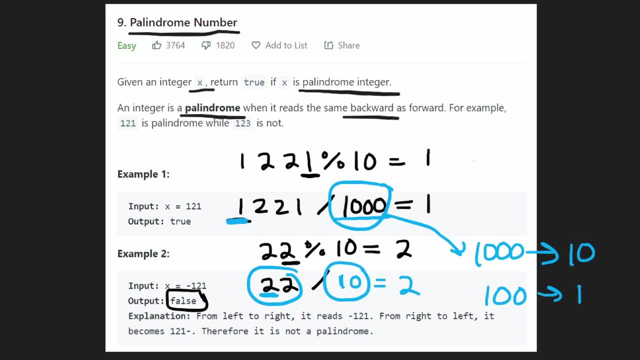 hundred went to being one. so on each iteration, this value, it could be really big, right? it could be 10 000, right? every iteration it's going to lose two digits. so it's going to go from being 10 000 to maybe being a hundred and then once again losing two digits. it's now just going to. 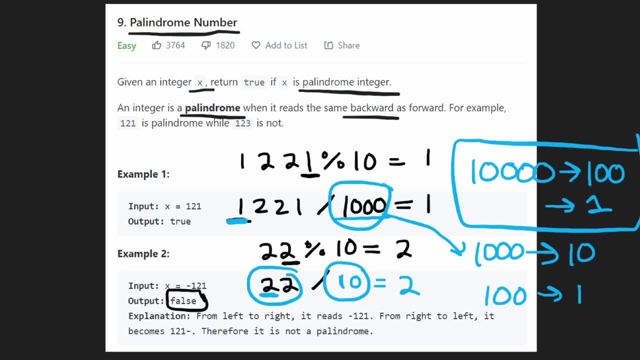 be one until the loop has basically been done, executing once we have no digits remaining. so i hope that this is helpful, because this is the math that we're going to be doing, and the rest of the problem is that we're going to have to do it again. so we're going to have to do it again. 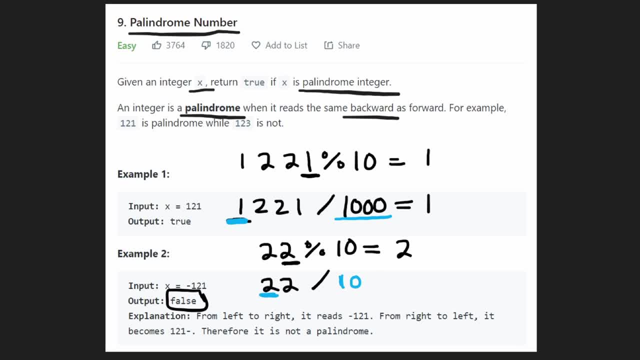 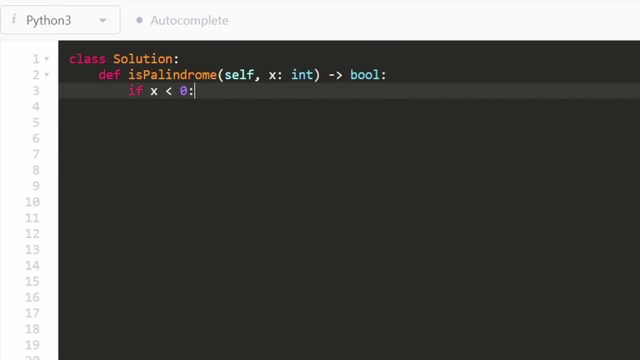 so let's jump into the code now. okay, so let's dive into the code now. we're given an input value, x, and the first thing we're going to check is: is this value negative? is it less than zero? because if it is, then we can basically return false immediately. right, that's what we discussed. 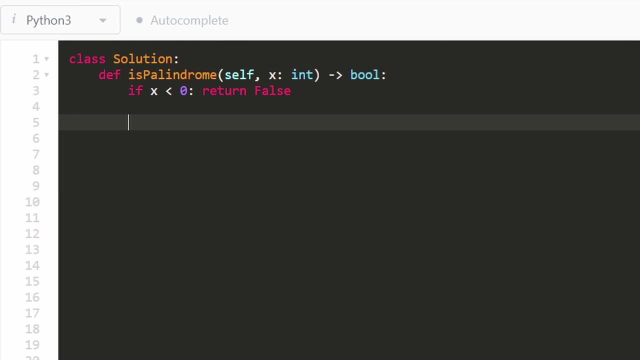 from the second input example. the next thing we're going to do is basically come up with that divider value that we were using. remember that value. that could be a hundred, it could be a thousand, it could be anything right. initially it's one. we want to know how large the value. 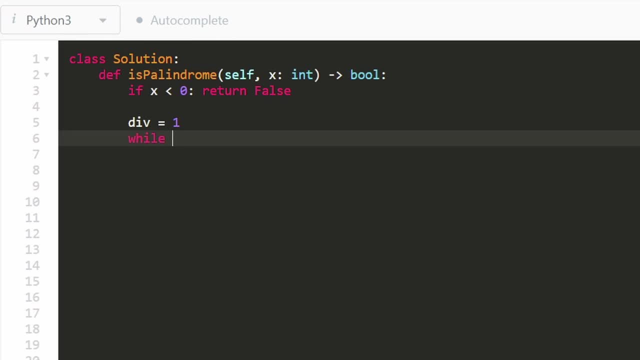 should this be so, how are we going to determine that? well, basically, if x is even greater than 10 times the divider- and not just greater, but maybe greater than or equal, if it's greater, then that means we're going to continue to increase our divider right, basically divider. 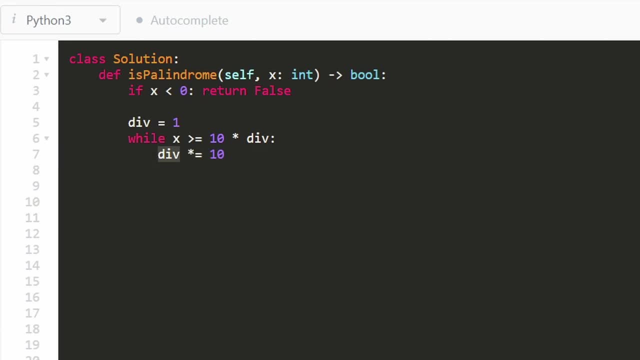 multiplied by 10. right, because we're trying to get the most significant divider that we can, that is still less than or equal to this x value. right, that's what we're trying to do. right, if we have a value 121, we want to get at least a hundred. right, if we have 121, one. if we have a value 1200, then we: 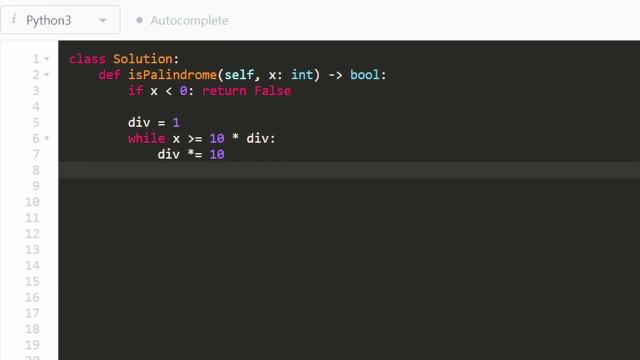 want to get to at least a thousand. right, that's what we're trying to do here with this while loop. once we have that, then we're ready to roll with the rest of the algorithm. we're going to check. okay, while x is non-zero, right, we're going to keep comparing the left and right digits. 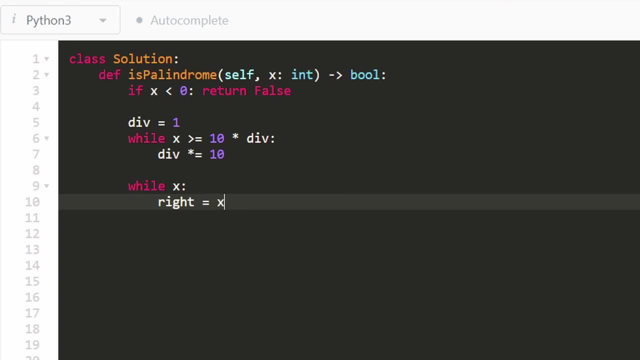 how do we get the right digit? well, remember, all we have to do is take x, mod it by 10. how do we get the left digit? that's slightly more difficult, but we can still do it. all we got to do is take x and divide it by the div, the divider value that we determined up above. i'm using two slashes. 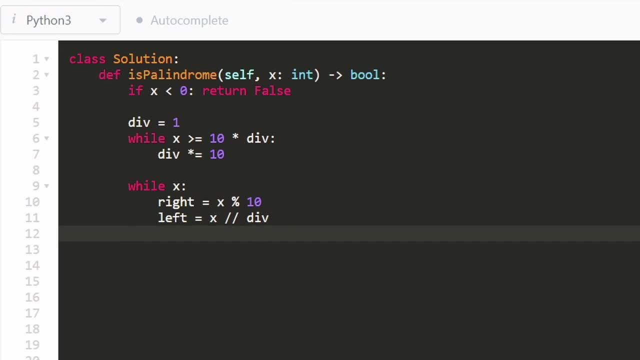 because in python this is how you do integer division. and once we have these left and right digits, what are we going to check? well, we just want to know if left does not equal right, then we can return false. so now we want to chop off the left and right digits. right, because we just 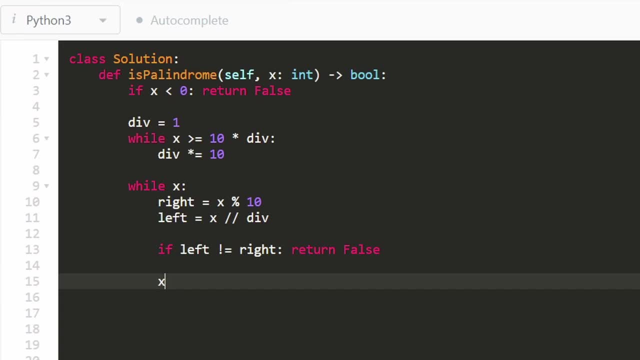 used them up above. how do we chop off the left digit? well, you might remember, if we take x, mod it by the div that we determined up above, that will chop off the left digit. so now we chopped off the left digit. how do you chop off the right digit? well, basically, take this integer division by 10. 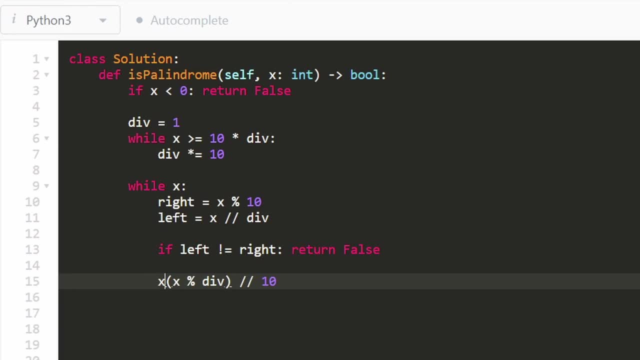 and then you're good. so we chopped off the left and the right digit with this single line of code that i just showed you, and remember, last but not least, that divider value up above div. we don't have to update this as well. how do we update this? well, every time we just want to chop off two digits. 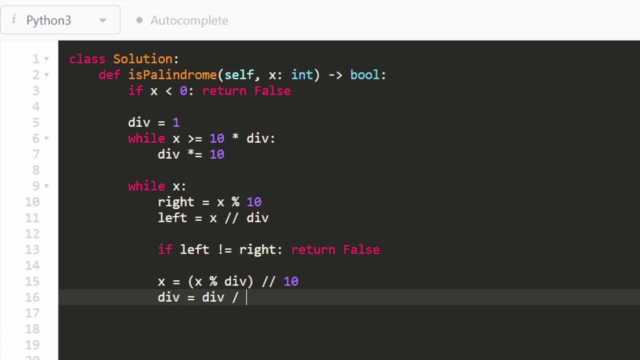 from it, right? so how do you do that? we'll just take div, take itself, divide it by a hundred. that will chop off two digits for us. and, believe it or not, this is the entire code. once we're done with this while loop, we will have successfully determined that it is a palindrome, so we can 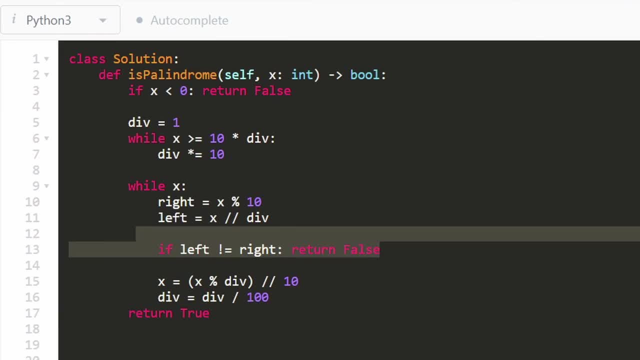 return true out here. we return false inside if it's not a palindrome. and this is the entire code and i'll run it to make sure it works and it is efficient. and yes, it is, and we're going to pass the divs in from the left digit. so we're going to take the right digit and we're. 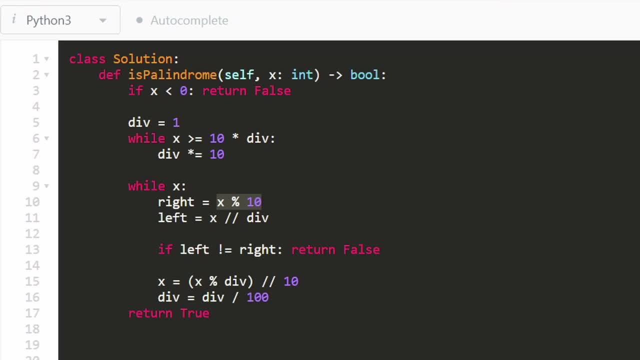 going to paste it in the right digit. we are treating this as the string of nodes, and i'm going to use my dog talking, so i'm going to show you how to do this. and one last thing i want to mention: you can actually take these two lines of code up above, left and right. we don't actually. 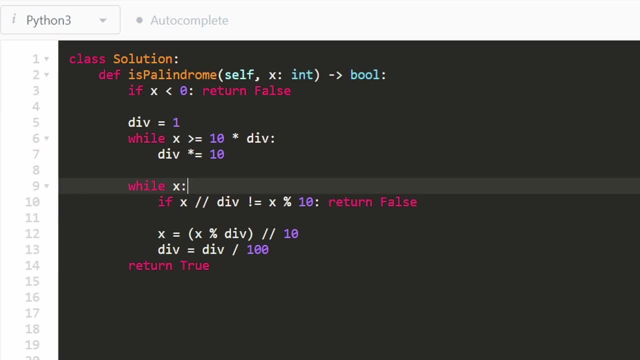 need variables for them. i just used that to kind of make it simple for you. you can take the right value and then cut it and then just paste it in here for this condition and take the left value, cut it and then paste it here, and then we can get rid of those two lines of code. 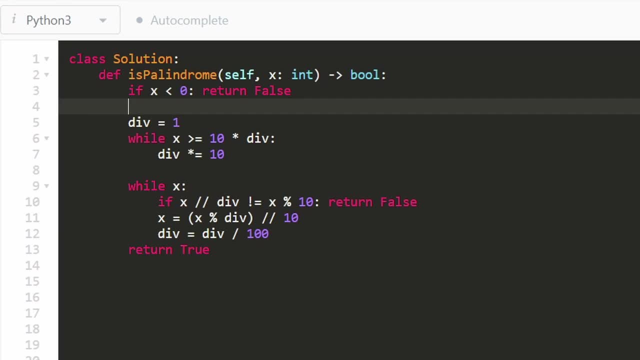 and you know, then the solution looks pretty short and easy. it's definitely not as easy as it looks. i would say. this is this follow-up portion at least is a medium problem, because it's not sharp enough, not easy to come up with, but I hope that this was helpful. If it was, please like and subscribe. 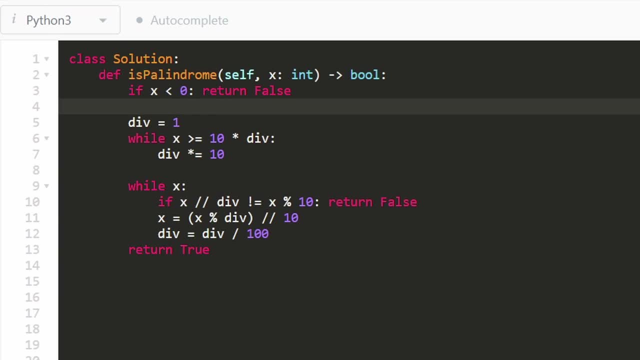 It supports the channel a lot and I'll hopefully see you pretty soon. Thanks for watching.